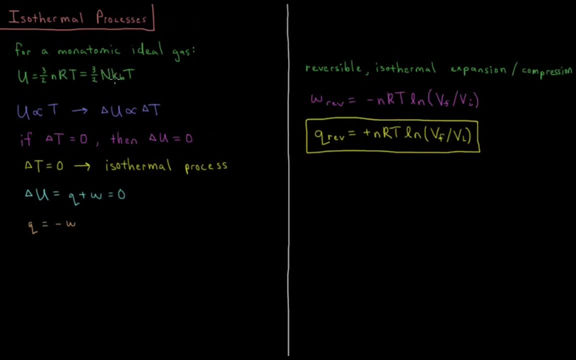 temperature or number of particles. times Boltzmann, constant times. temperature nR equals nK, So that's the translational energy for a monatomic ideal gas from statistical mechanics. So what we see here is that for this particular type of ideal gas the internal energy is: 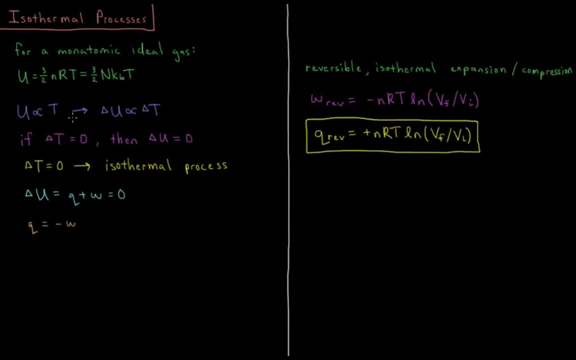 directly proportional to the temperature. So during some process the change in internal energy is going to be proportional to the change in temperature. So if we have some process where the change in temperature is going to be zero, then the change in the internal energy of an ideal gas is also going to be zero. 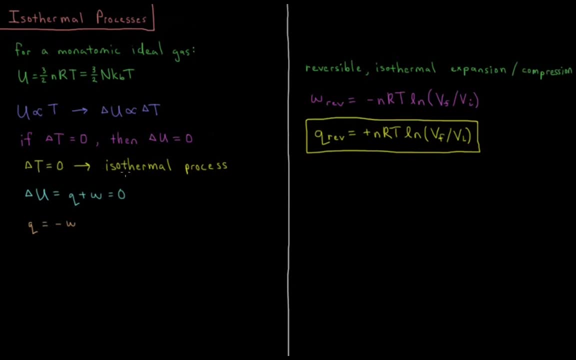 So processes where the change in temperature is equal to zero are called isothermal processes, Iso being the root word for same and thermal as it relates to temperature and or heat. So we have that for an isothermal process If our temperature doesn't change. for an ideal gas, if the temperature doesn't change. 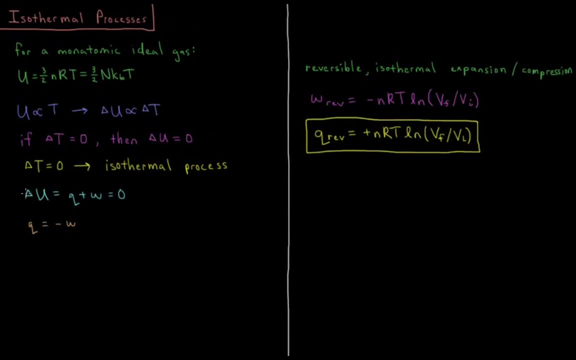 then the internal energy doesn't change. So the internal energy change of a closed system is going to be the heat plus the work that occurs during that process, which we've now said is equal to zero. So thus the heat that occurs during an isothermal process is equal to the negative work. 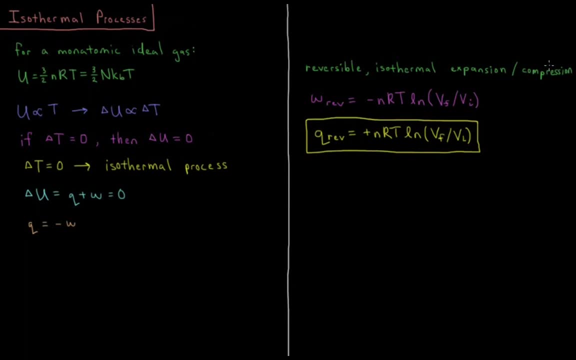 So for a reversible isothermal experiment, we're going to take the heat and the work. We're going to take what we're left with the heat, which is what we have here, and isothermal expansion or compression of an ideal gas. we showed that in the previous video, that 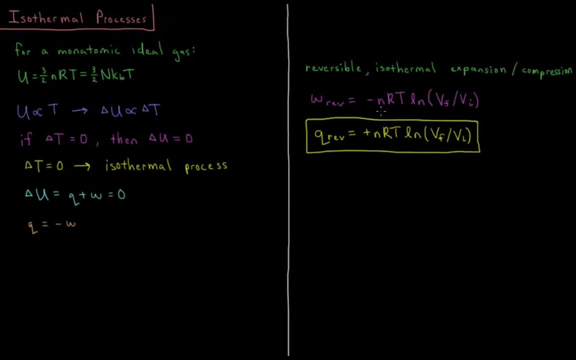 the reversible expansion or compression of an ideal gas. the work that is done during that process is equal to negative nRT. log V: final over V, initial number of moles, gas, constant temperature, final volume of system and initial volume of system. So the heat that it so we're. 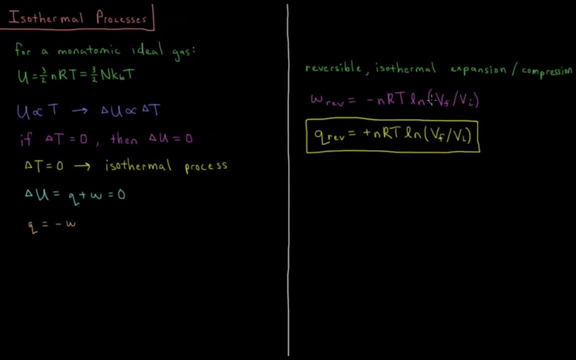 doing work. So whatever work we do is negative. nRT log V final over V initial. So the heat that we need to input into the system or remove from the system needs to be equal and opposite to the amount of work that the system does. So if the system expands and does work on the surroundings,